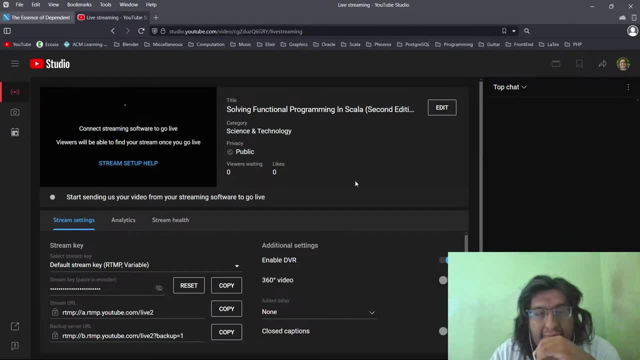 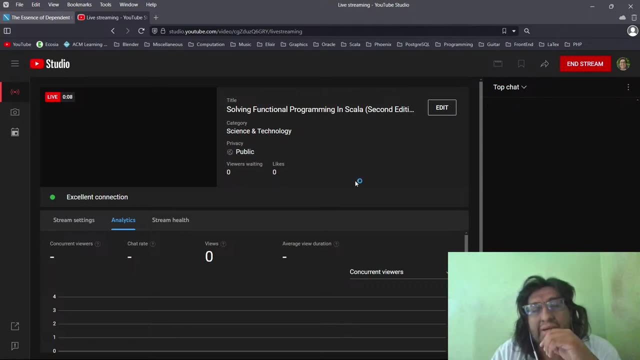 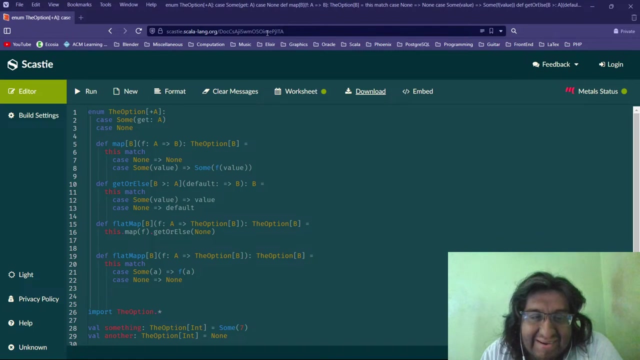 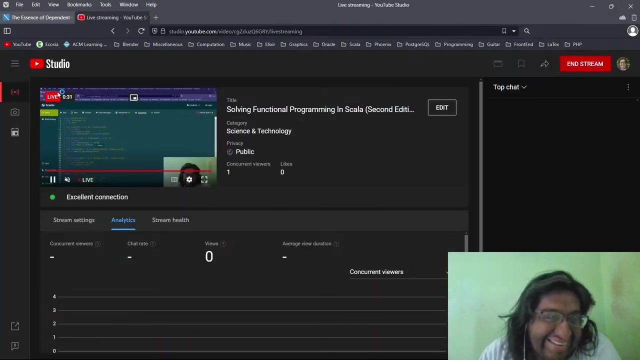 Good morning everybody. Good morning. Yeah, we are live 10 seconds And I did put this starter URL in the video description. You can, you know, give it a try. And before we start, you know, I have to tell this Yesterday the thing: if you are following this series, which is a little few people are seeing this video- Facebook. 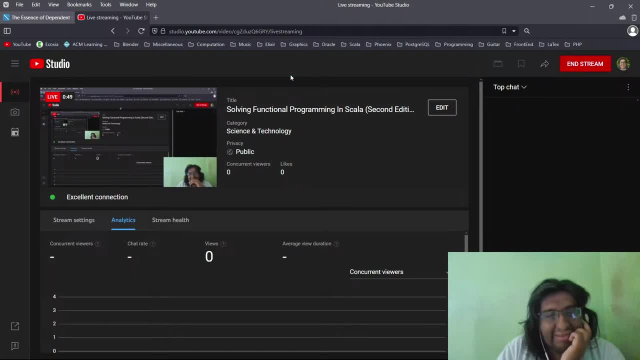 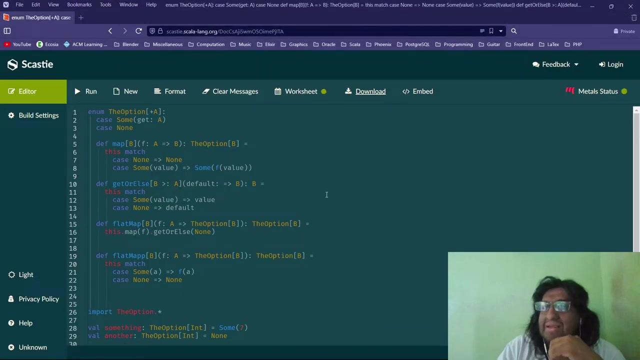 You know, yesterday things went nuts And I don't know. I mean, I choose to study Scala many years ago, many, many years ago, But I never committed to learning Scala because, for some reason or another, I never completed any. 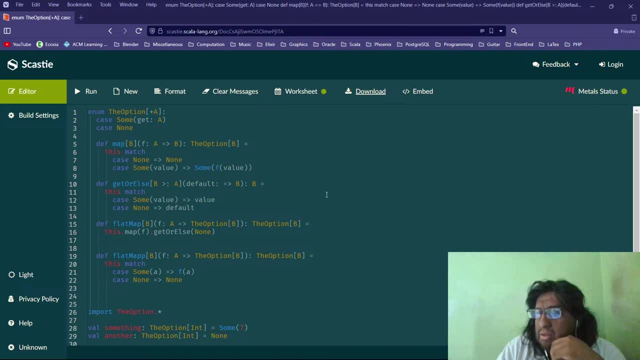 training to the end- That was changed two years ago- in which I have enrolled myself in effective programming in Scala, which I will be doing a review. It was, for you know, at last, one complete training course for me, But in I have, I discovered Scala And I choose to study, to study, to give some time to this language, because it seems to me that it's quite a product, you know, delivered by Martin Odersky and his team, And I I think it has the philosophy of this guy. 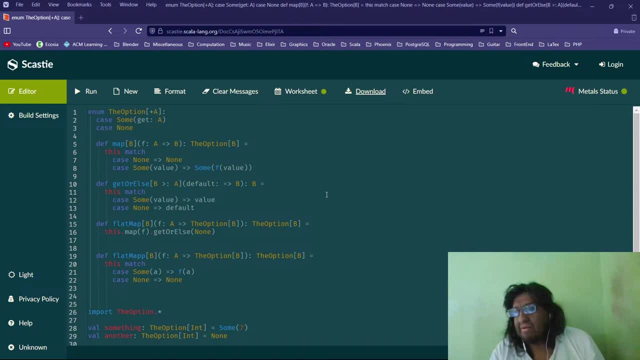 Martin Odersky and others And they, according to Martin Odersky, they were in their training. while they, while they were students, they interacted with Maurice Wilkes, the guy who invented Pascal, And the language is a good thing. I- I I didn't get a chance to study Scala. 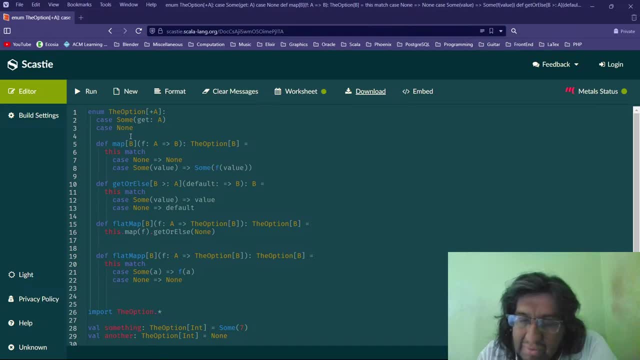 why W partnered with Martin I. I've tried many, many different things over the years and I got to know, to learn about- and I forget to know the Scarlet too. a, to be honest, Martin Odersky and others And they- according to Martin Odersky, they were in their training while they, before they, were students and I thought that it was a good thing. And after that, I, I, they- got to know and I forget to know this color too. I love to be honest, perfectly. 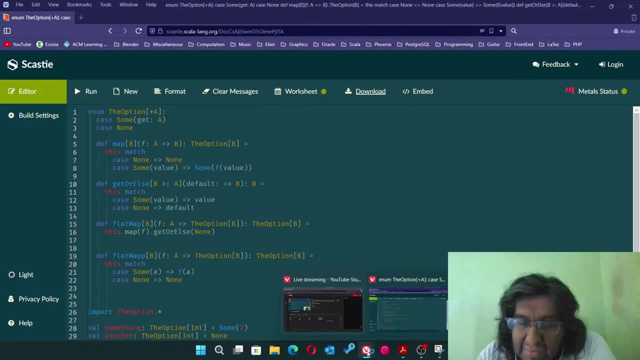 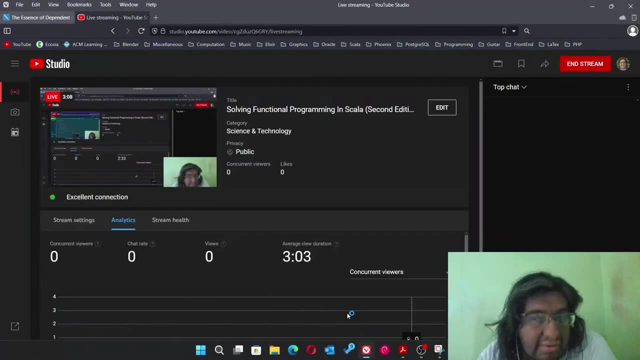 Martin Odersky and others out my attention. I noticed this session to see personal growing day, but it's still home to signalot always my attention. i So it's still escape. struggle and suffering. Well, not suffering and struggling, but to see a person who's struggling. 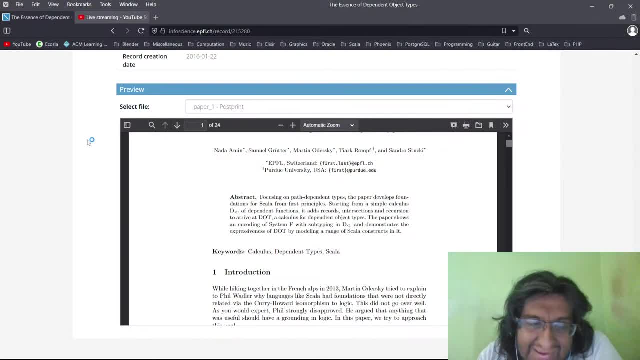 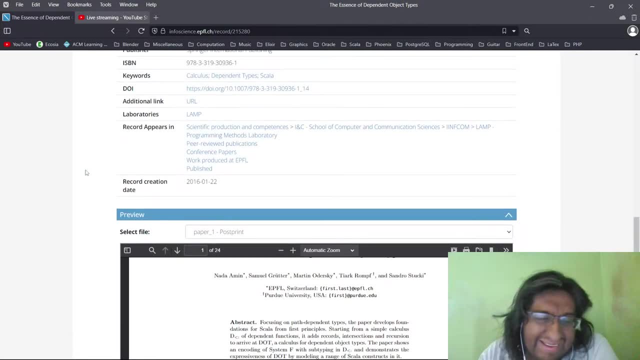 It's like one person. I don't lack to meet another person who's doing this stuff, person solving these problems in the book, but since yesterday the things were some kind of I don't know. I don't know what happened, with disgusting and with me to be blindly. 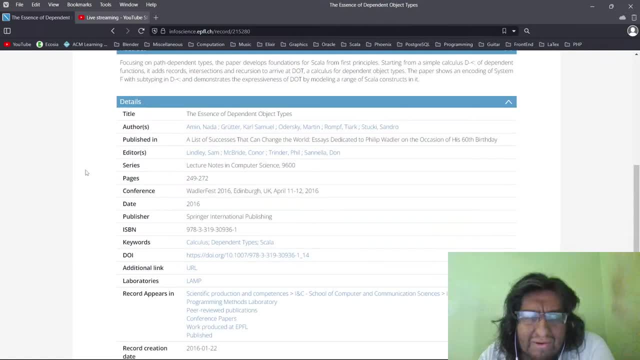 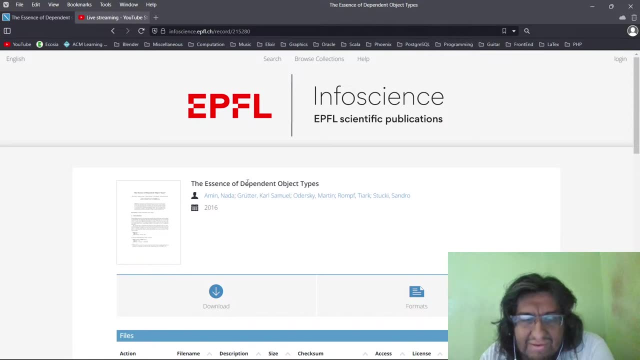 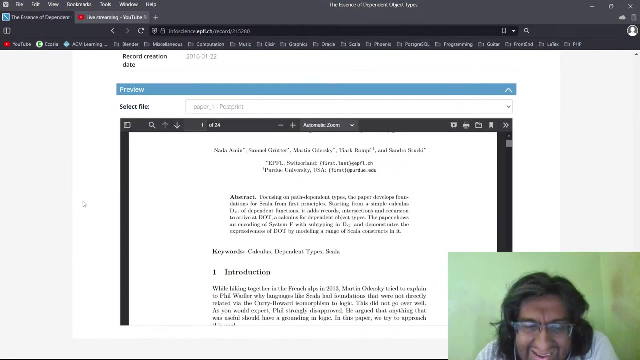 it was shocking. so today I looked for this uh paper. the essence of depending object types. this is dot dot and it's quite a rigorous thing that Scala has behind it. so that was people is trusting this and it happens with lots of programming languages. they have a 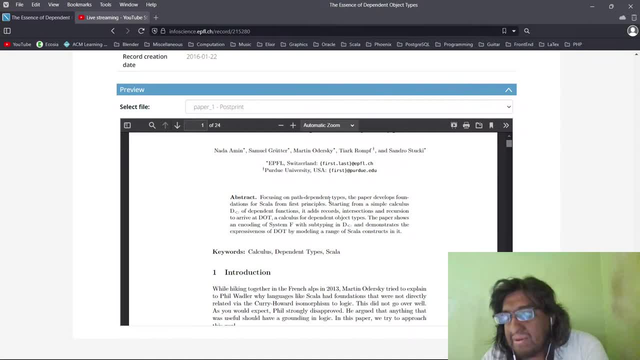 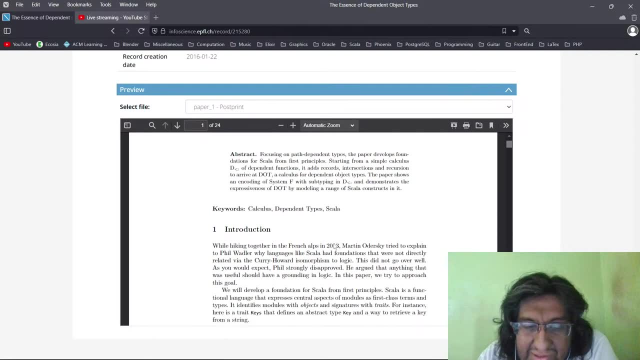 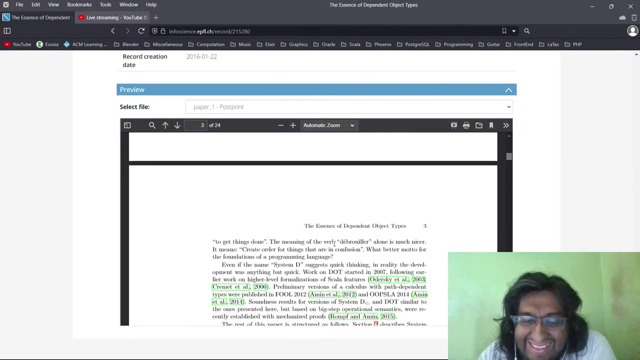 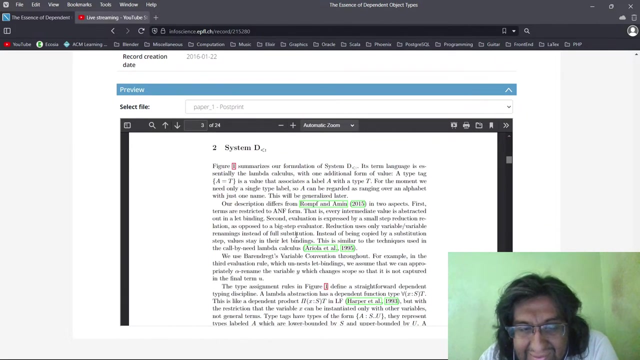 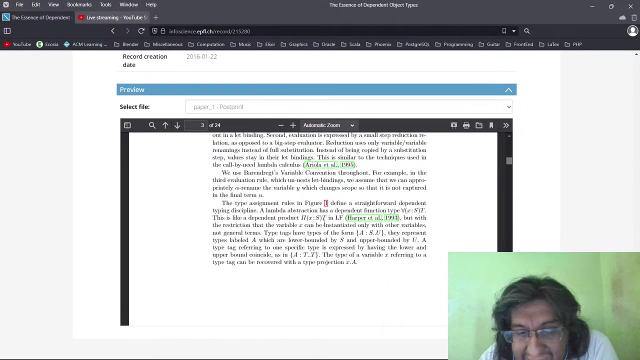 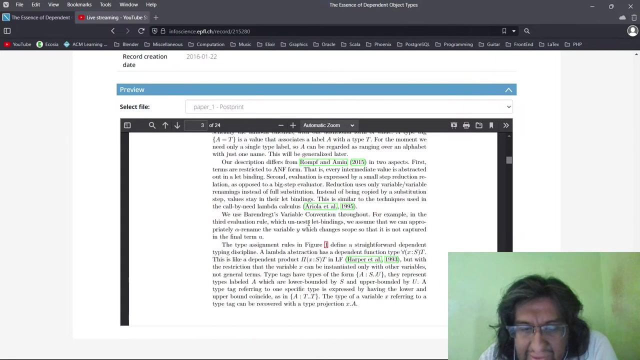 serious research behind them. Scala is one that has many years, uh, research. and look at this, how, how you can say that the compiler will fail to. you know, and there are some beautiful things around here, get things done. some translation of the world, uh, the system D I can, I don't understand. 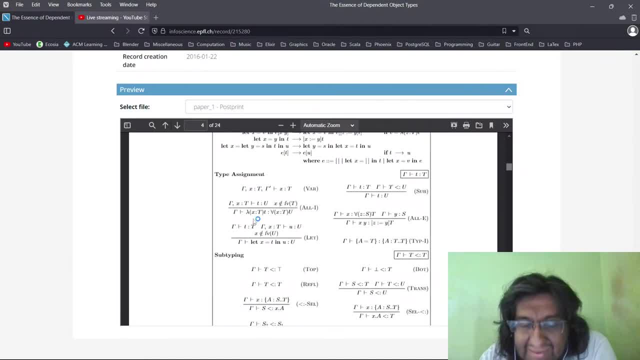 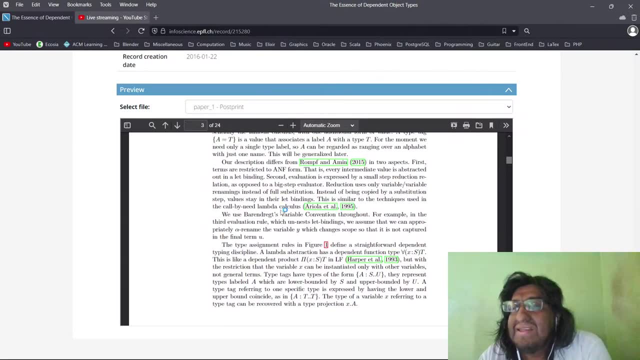 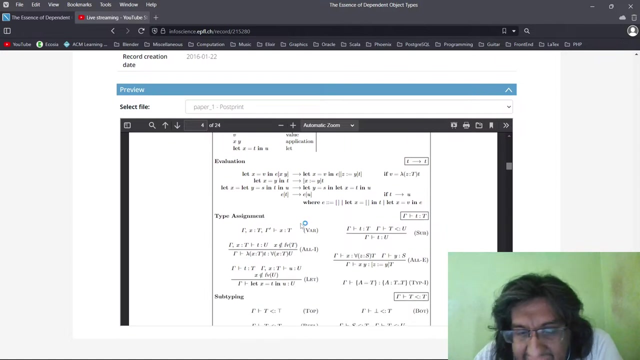 most of this paper. to be honest, you see a lot of this simplified. I don't get it. I just read the text. I am working my way and towards advanced topics in functional programming, but mathematically this is just like different stuff. uh, I recognize some of the symbols, to be honest, but um, 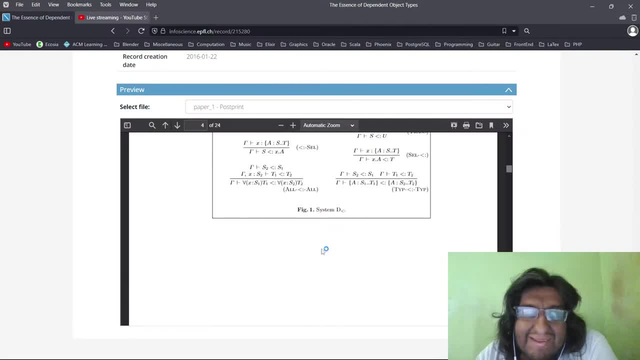 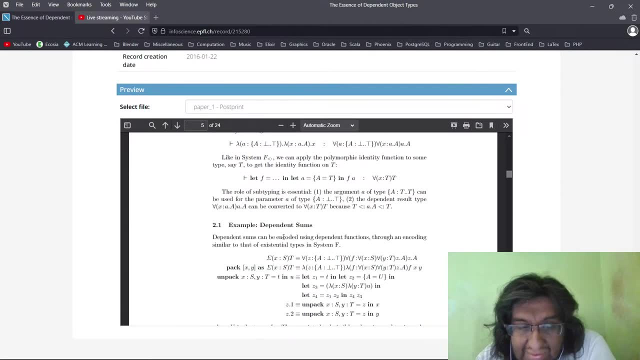 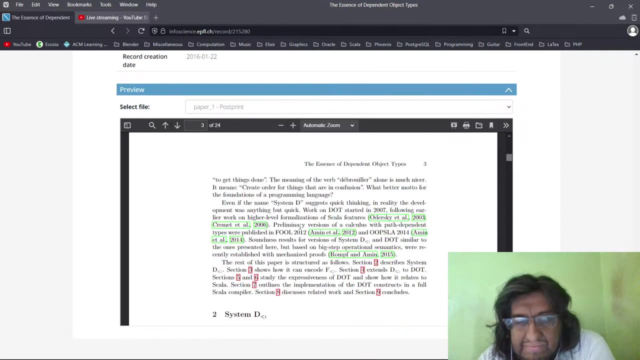 I don't know what it's expressed over here, and I don't know because I have in the studio this thing, because we are, I, we are all able to understand this stuff, okay. well, what I wanted to share in this beginning of this video is that you expect the 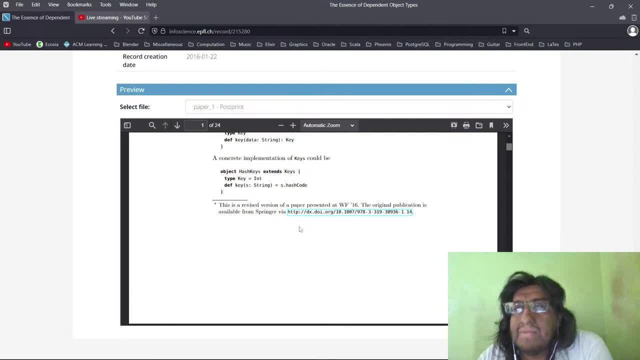 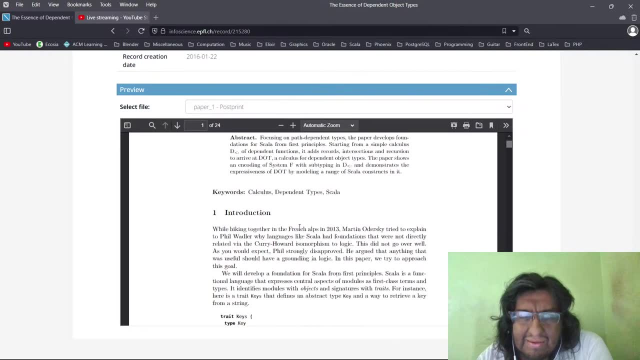 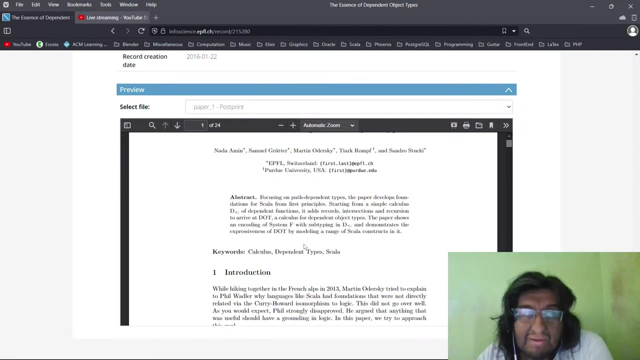 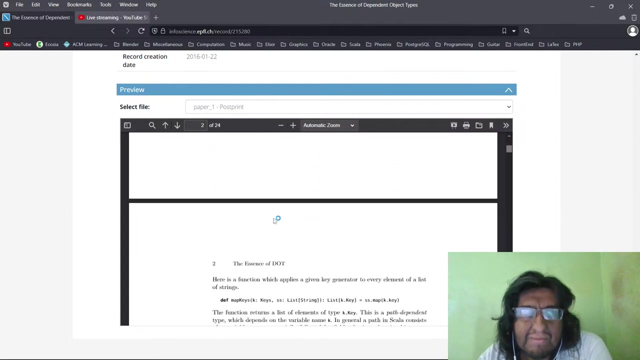 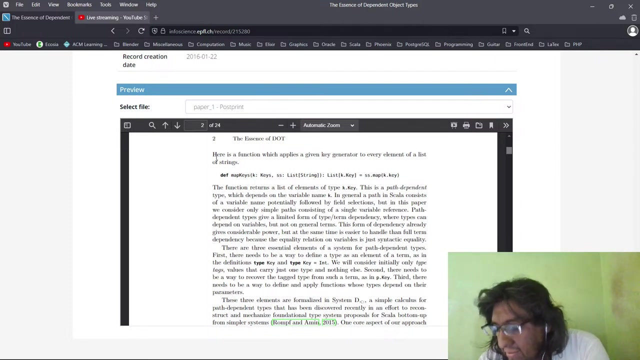 the trust behind having behind the trust of one compiler and despite with the work of this, like devote people to their crafts, you know the entire life, uh are invested in this stuff. when you say that okay, and but then again uh still use, we, i suppose we shall have some preservations. i don't know. 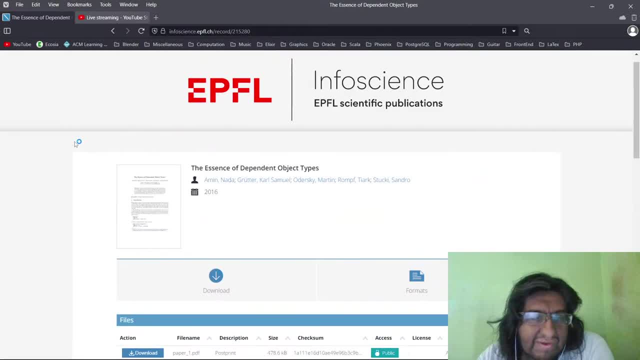 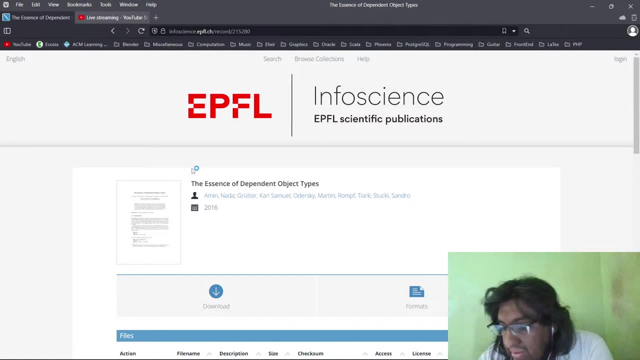 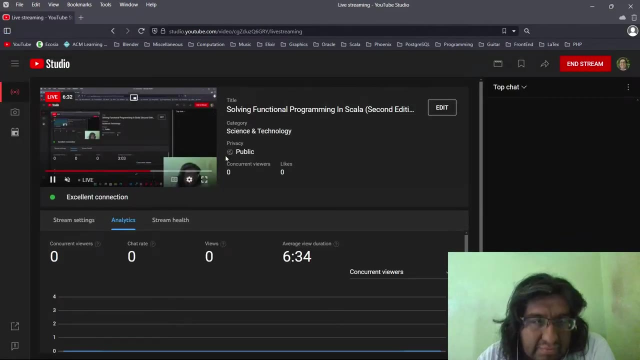 i? i don't know. you can search for this on your own. you know the essence of the pending object types, because i didn't put this in the in the video description. don't close in this tag now. now, in terms of time, i'm just giving myself for today's exercise. 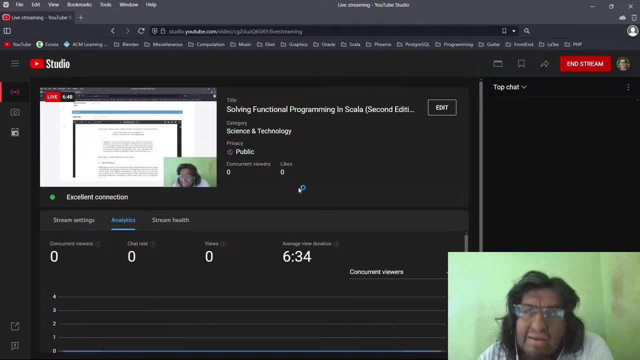 15 minutes, uh, 20 minutes at most, and if i can come up with a solution, or or things are going crazy, i'm not, you know, switching to this. i'm not, you know, switching to this 15 minutes at most, and if i can come up with a solution, or 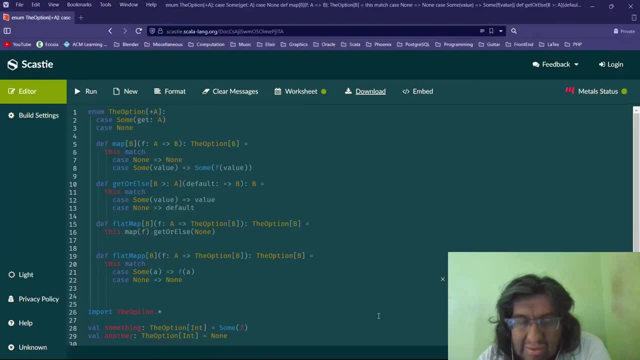 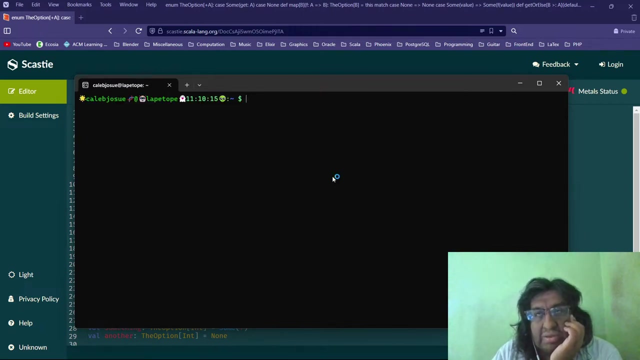 or things are going crazy. i'm not, you know, switching to this. i don't know, like yesterday that we were uh opinion-based in trying to lower. we'll just end the stream and probably work the solution in here on deviant and then presented the conclusions like uh when we did, but just in the concat. 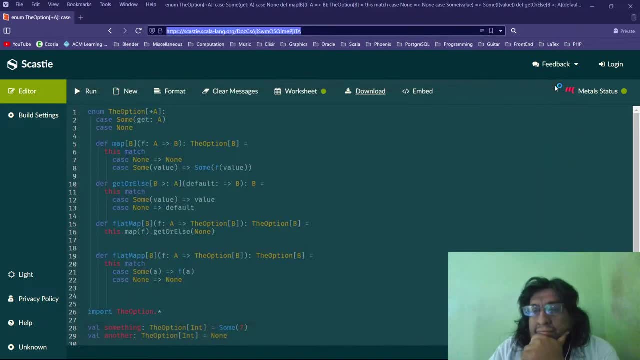 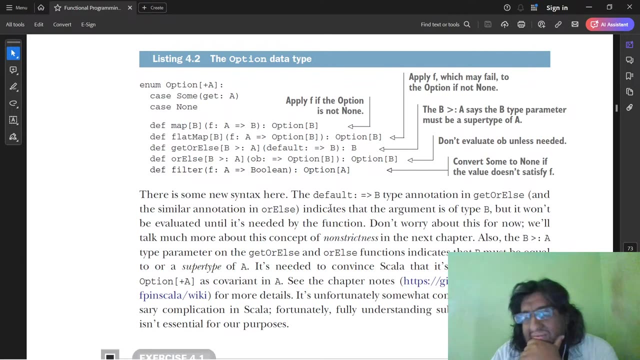 and then presented the conclusions, like uh, when we did, but just in the concat exercise. and then presented the conclusions like uh, when we did, but just in the concat exercise, you know. so, yeah, let's start now and see we can work a filter and it says: convert some to none if the value doesn't satisfy s. 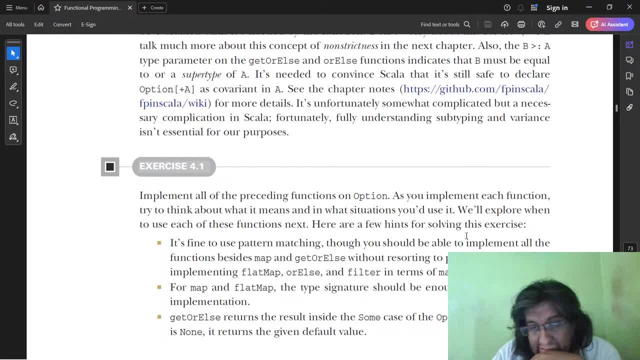 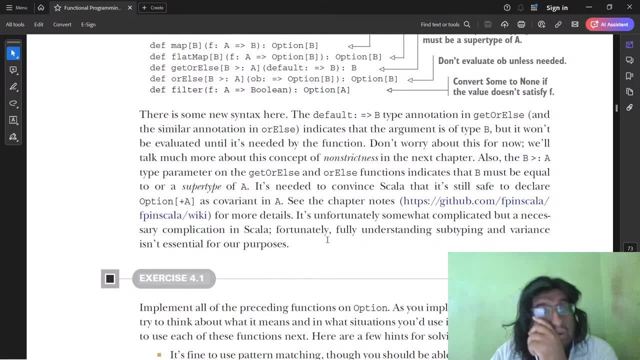 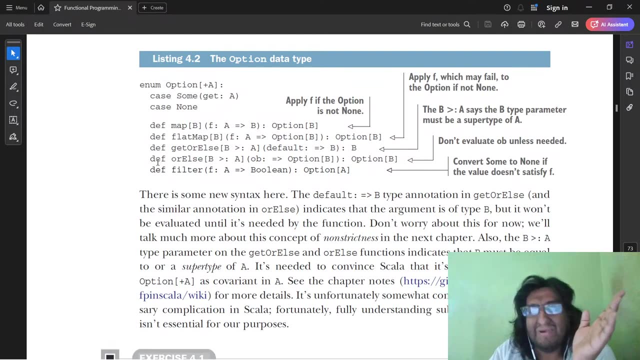 and again, if you tell it's, we are invited to try to implement filter in terms of map and get, or else we will give it a try. but again, i'm not, i'm not crazy about at this point, after what happened yesterday, but we'll give it a try. 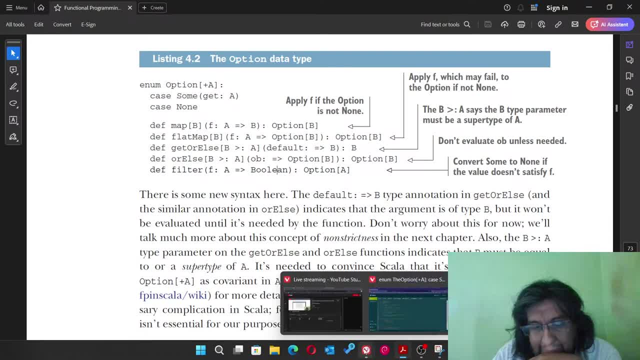 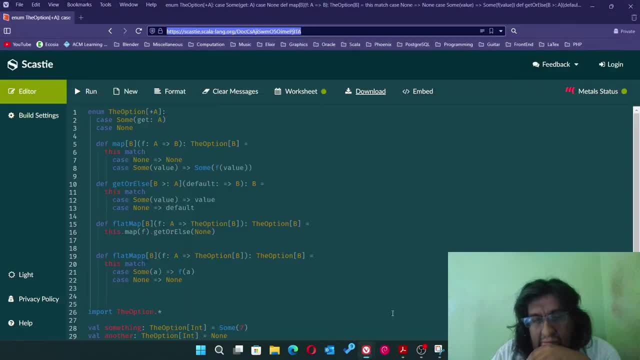 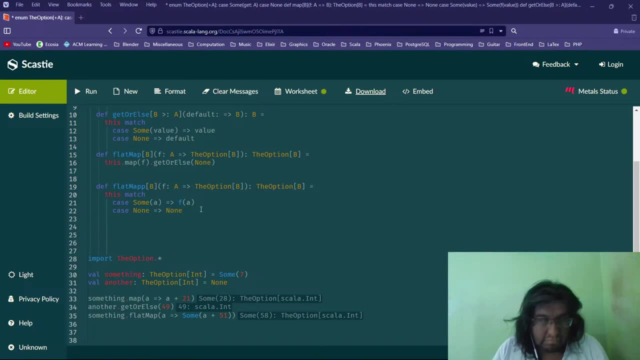 okay, we are copy and pasting this. uh, it cannot plus 20, 30 minutes, and that's all. okay, i'm pasting the definition. you should. you know what. let's use the flat map pp that we have over here. okay, and first let's demonstrate. 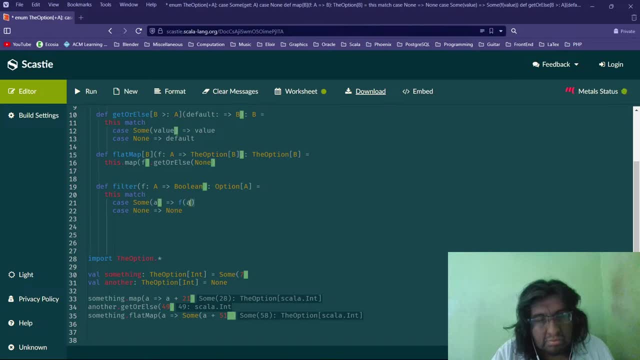 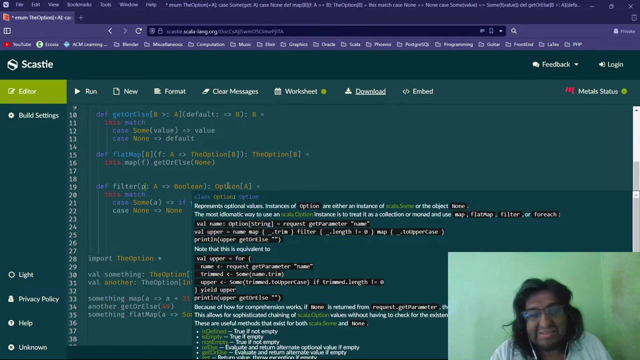 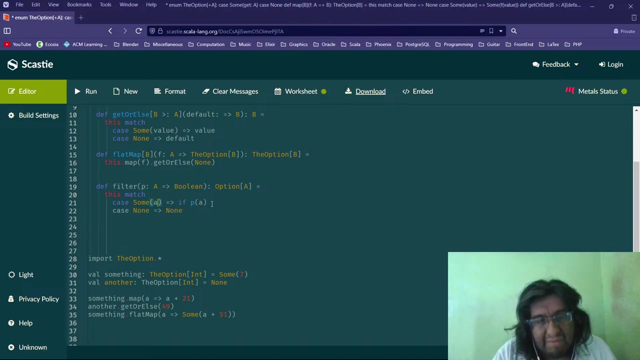 the thing with pattern matching. if um p of a, where is p? i like to call this p because there are predicates, but there are still functions. so f is okay, it's great too. yeah, p of a. yeah then, and we have options, but ours is the option. 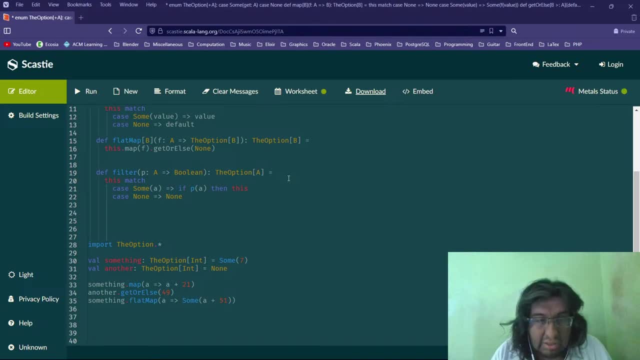 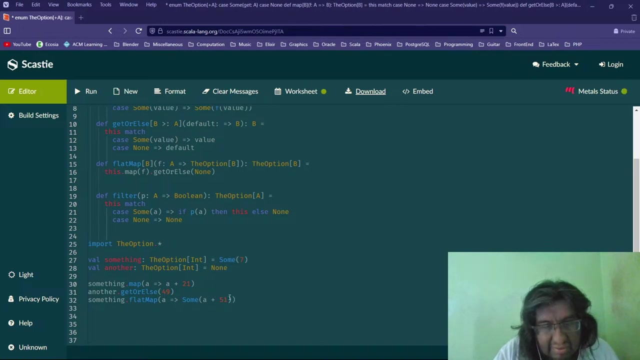 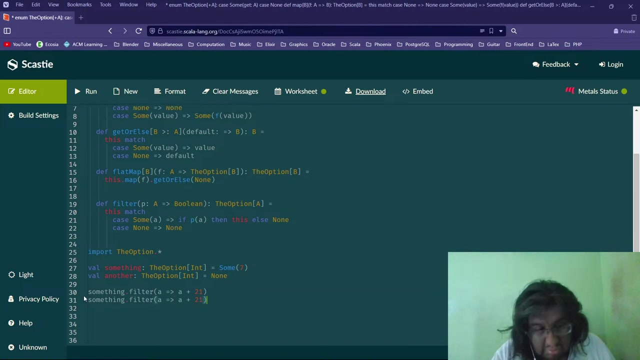 i will return this if it doesn't work. i think none. i suppose that should do it. and the option in seven? okay, let's uh get rid of this. another: it is the filter filter. okay, something, filter filter. we need to pass a predicate. can we do something like this? 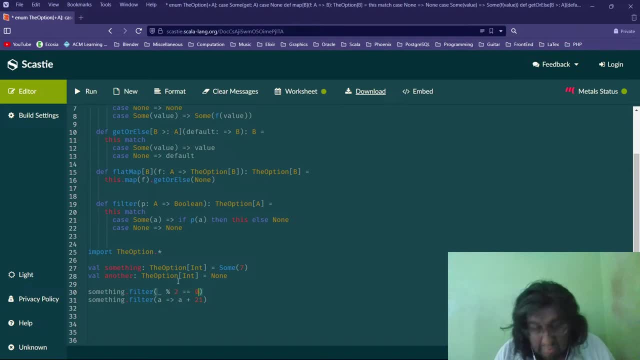 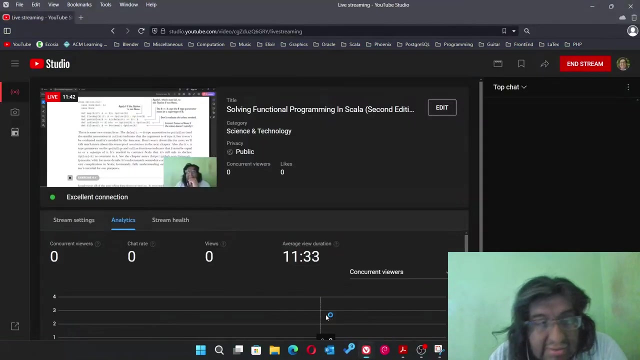 not true, because here we are asking if, if the number, if the option contains a value, that is even so, in here we expect none and in here we expect seven. sorry, we are uh, in here, okay, we have seven, seven, seven, seven, seven, seven, seven. in here we expect seven and in here we expect none. let us see if we are here right. 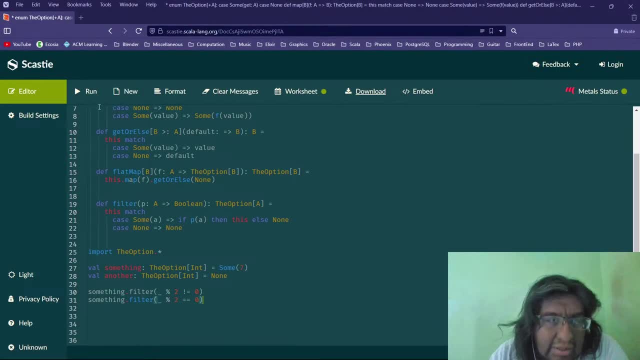 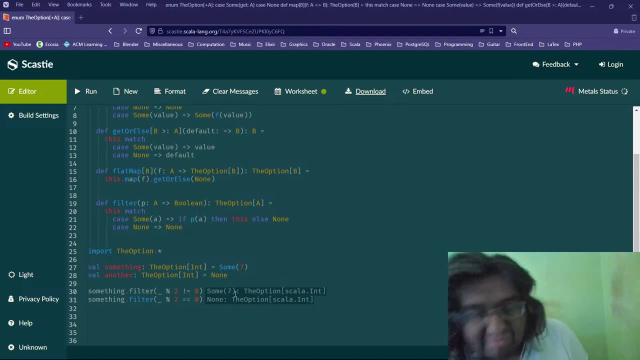 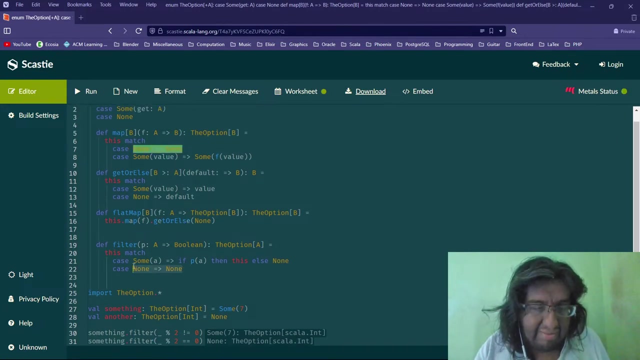 i thought 12 minutes, i'm not sure. okay, some seven, none, i said seven, i know, but hopefully you understand that we are returning an option. but the thing is mechanical, you know, without even thinking we are, you know, and we are invited to write this in terms of map and get all else. so i will give it a try for sure. 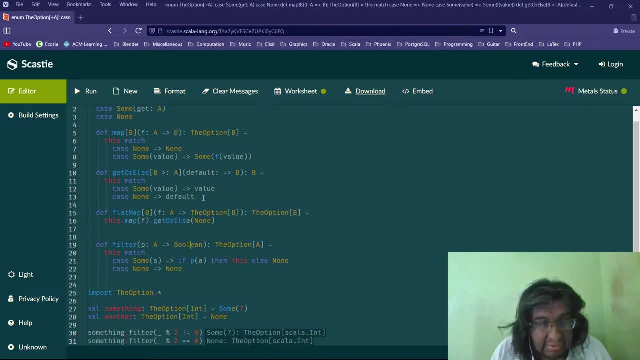 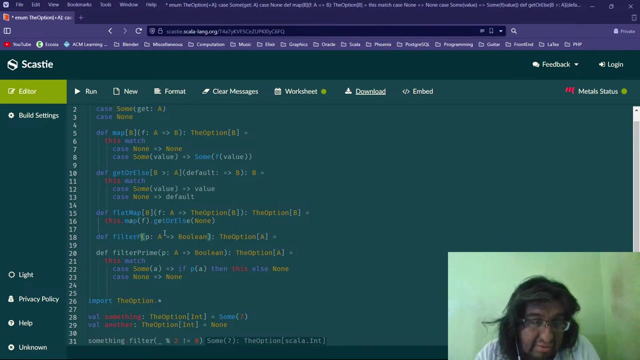 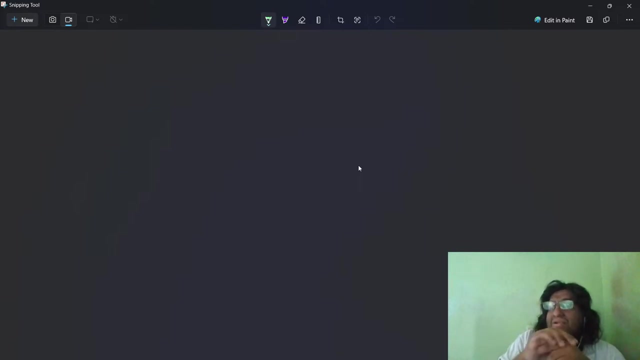 so i will solve this: use the filter prime and then we find another filter with this same type signature over here. i'm calling only filter and i, i have me in my chalk. uh, talk about you have. uh, probably i should think first to solve the problem. let the explanation to be: this is the option. 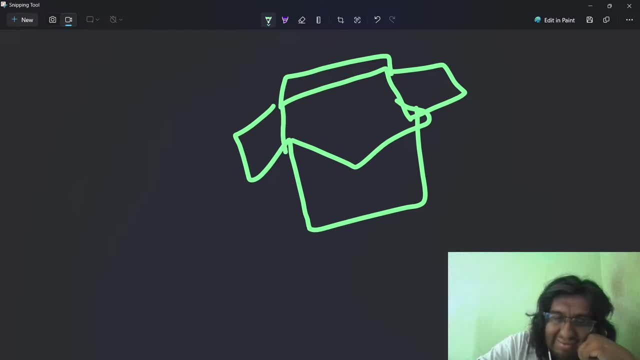 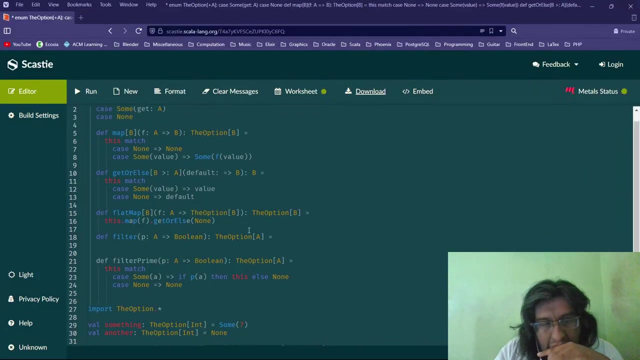 so let's see. let's see q, and inside here there is a number, but it's inside the option. probably this is for questioning to evade, avoid thinking. yeah, this is a depiction of the option. okay, now for some real thinking. let's uh, maybe we use theаются. 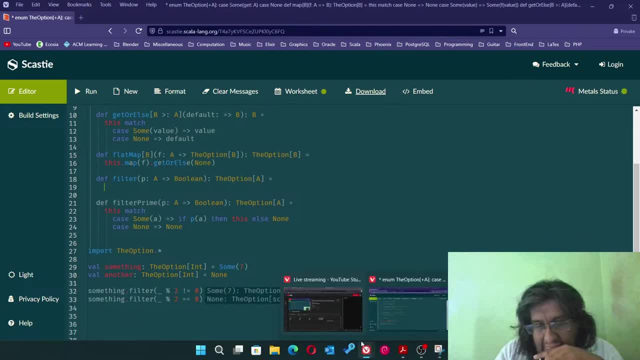 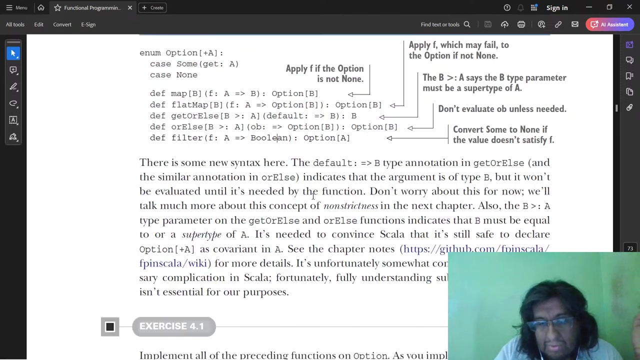 let's start with some things. uh, you're gonna try. well, this- sorry, this is real thinking too. now everything is okay and we should be happy right now. okay, don't get stressed if you are writing this, but now the invitation is still open in the book to implement a filter in terms of map target. 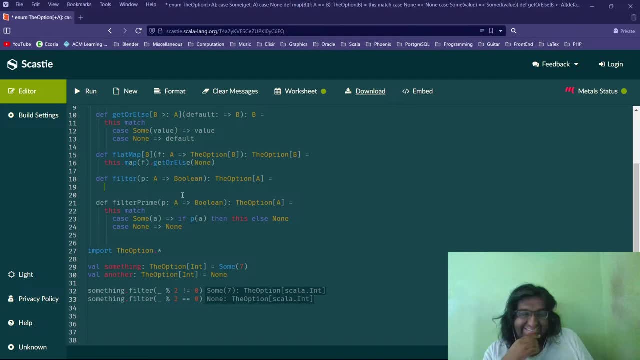 how should we proceed with this? we are again in the same place as yesterday, which brings me to the next question. yesterday we did have plasma pp with this pattern of shows that was failing. was the line in that function, that particular line? so i don't know what happened. 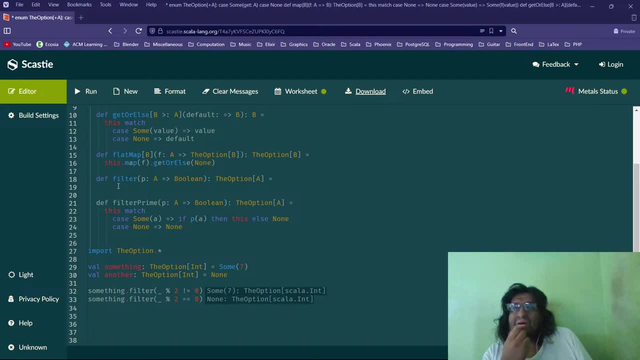 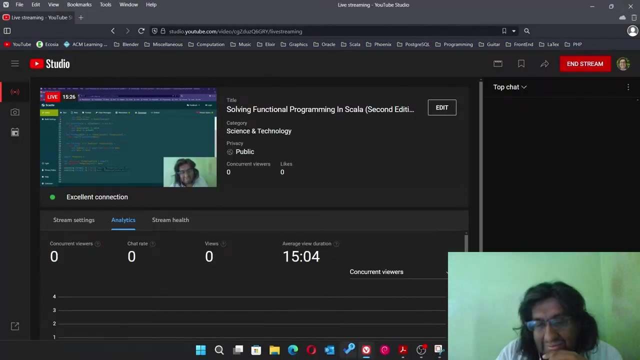 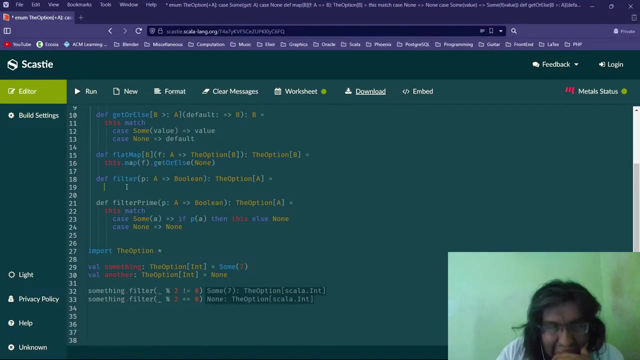 which brought a lot of questions to ourselves. uh, you know, okay, let's avoid, uh, let's try to avoid the thing issue. all right, can we do? well, it seems we should use map and get or else. yeah, look in the powers, hello else. what if we use get or else at the beginning? 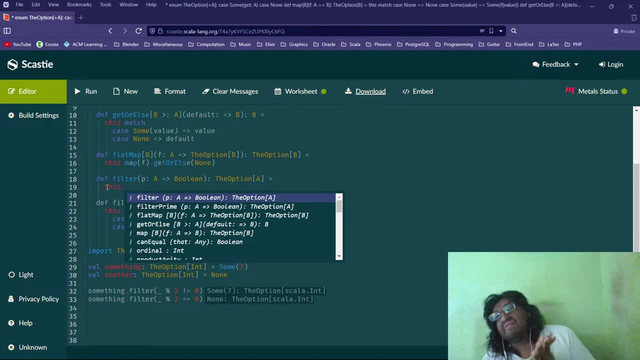 which, if we use, if we use get or else, at the beginning we will need, uh uh, a variant which i haven't test. if i'm yeah, an expression can be, can be an argument of our functions. yes, but we are not doing that, so let's go with map. 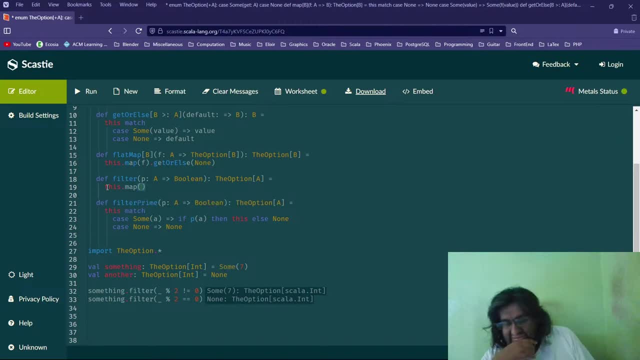 and again we are in trouble here because we need a function. again we are receiving this a and if i'm not sure if this is going to work, to be honest, here's a and this else, no, uh should be. should this be enough? again, we will be returning the option, the option b, that's yesterday. 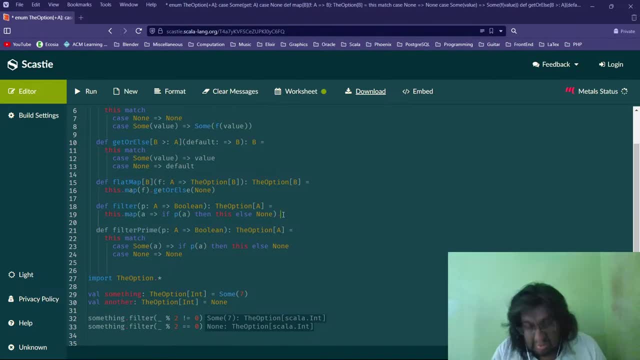 well, anything can happen at this point of time. you know, no say, yeah, i don't know. no say in spanish is: i don't know in english. let's hope for the best. no say in spanish is: i don't know in english, let's hope for the best. 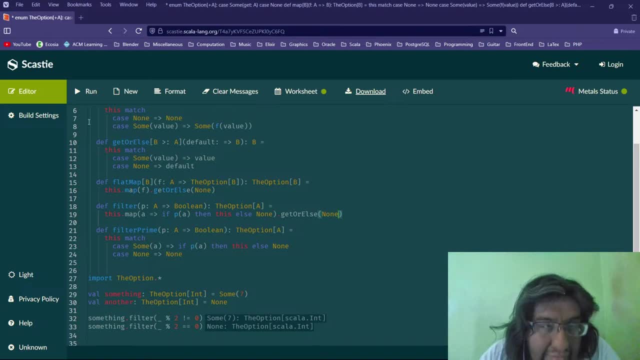 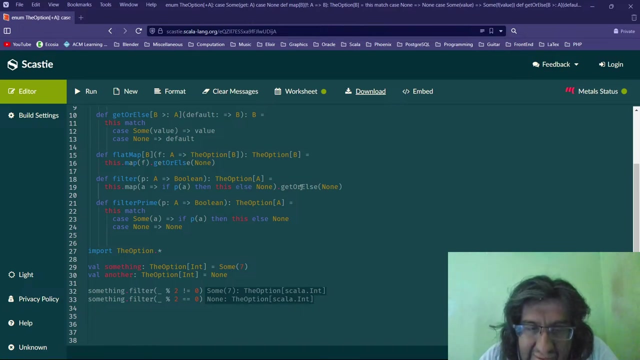 let's hope for the best. i feel that it's not in spanish. if, if you, you have made a mistake and we are done, thank god, thank god, but i have the question, but i have the question, but i have the question: if, if, if you know, we have known as known, whether 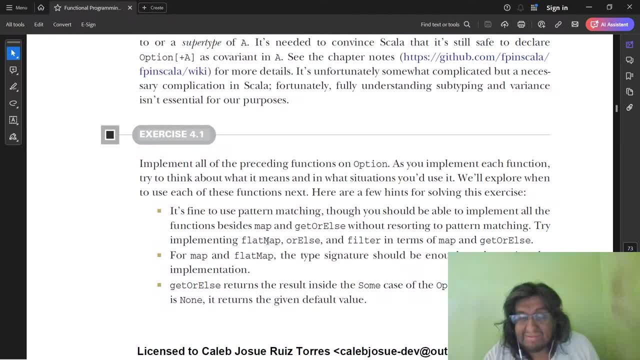 we are mentioning known twice. we are mentioning known twice and at the end, because i don't want to risk myself to see the answers by looking for some issue like that happened in the fault function. We were looking, we were getting again strange results in. you need to see that video from. 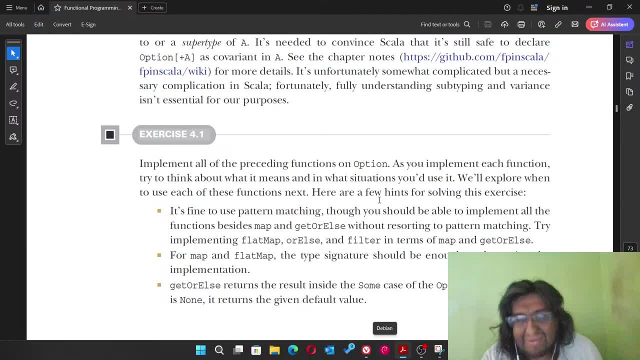 the REPL itself. You know, the functions were like. I don't know if I typed it wrong in the wrong way in the wrong way. After looking for some related issues with that function, we ended finding that the official GitHub repository contains most- most, I suppose, I suppose- all the type signatures for the. 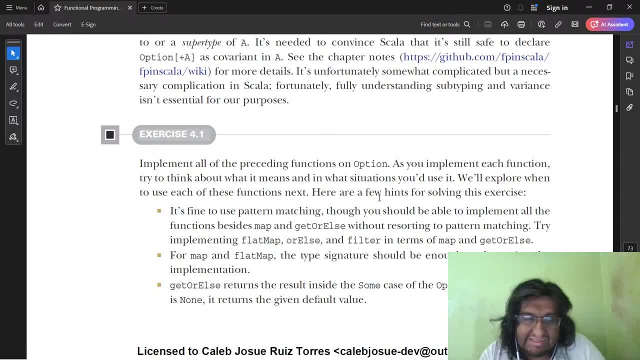 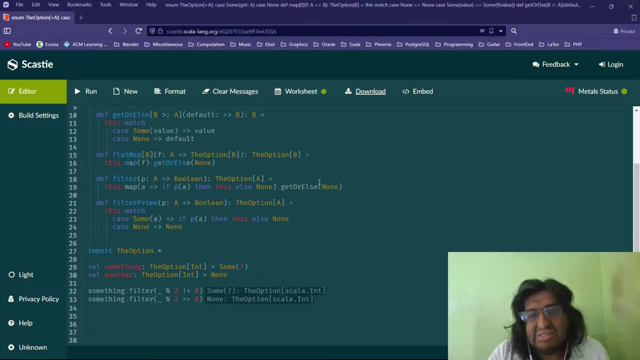 exercises. So only after we finish this chapter I would like to come back and look for filter in terms of map and get the results to see If the authors have another expression different than this. But for now, we will save this URL and see you tomorrow. starting from here to the final, 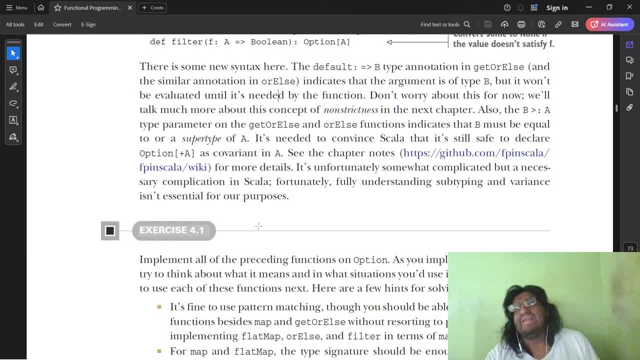 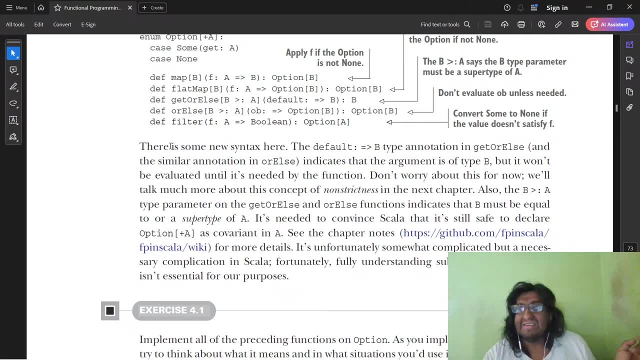 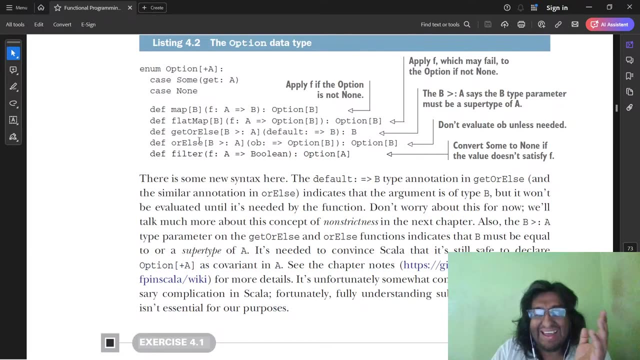 little exercise And it depends of your level. It could be, It could be, It could be. I would be like I don't know. Very straightforward. I mentioned yesterday some characters related to the functional programming area. Could be like I don't know. 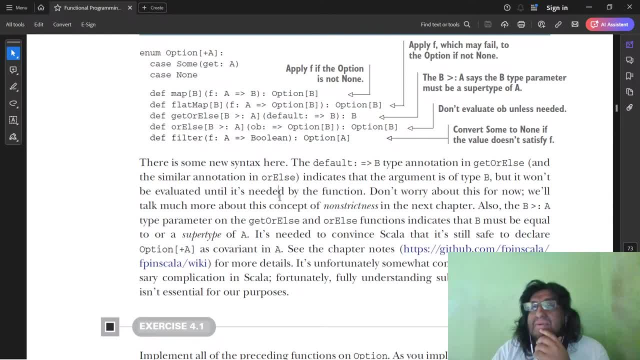 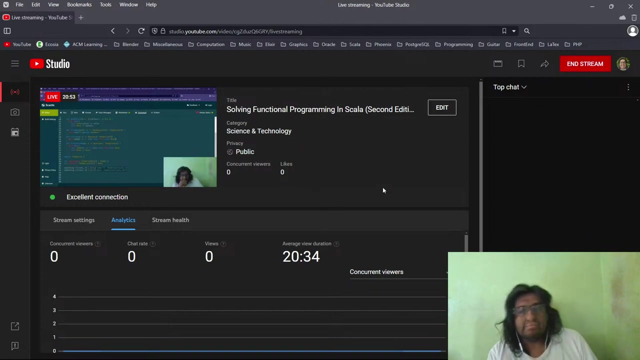 Very straightforward and If you are in your intermedia- intermediate journey and retaking this after some after bit challenging, especially when you combine the functions and the type, variables are very important, some kind of algebra in here. that's it, guys, that's it fellows, we are still live. thank you very much for watching this video. if you see. 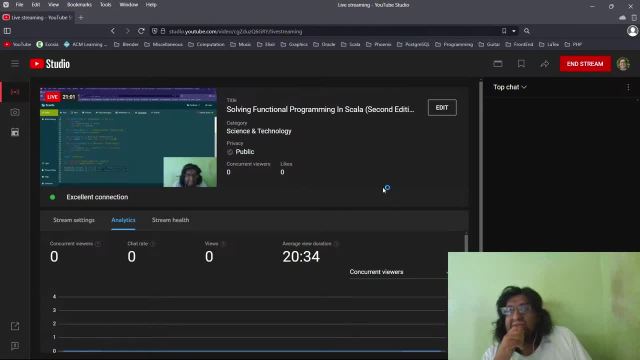 this in the future. i don't have anything else to say for today. in terms of office of functional programming in seattle. i will probably will blow up another video. take a look at the channel for other content. take a look at my website. have a great day and see you tomorrow, with the grace of above, lord. 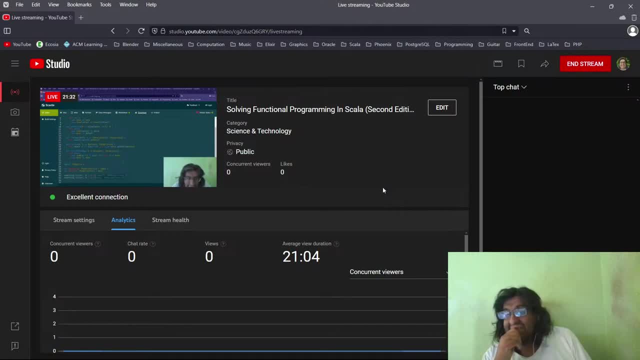 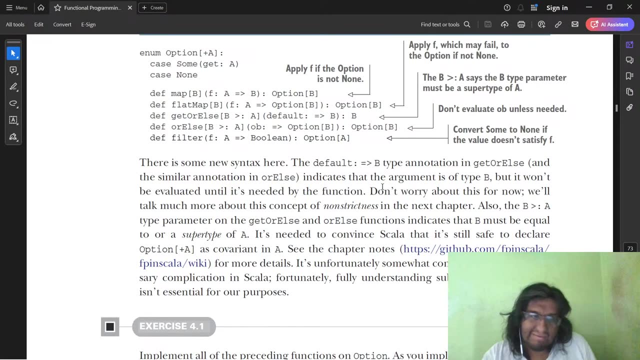 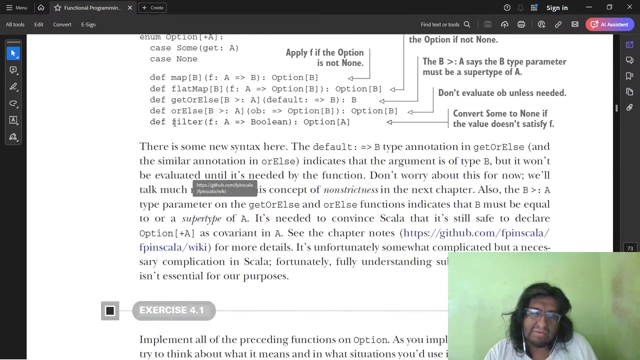 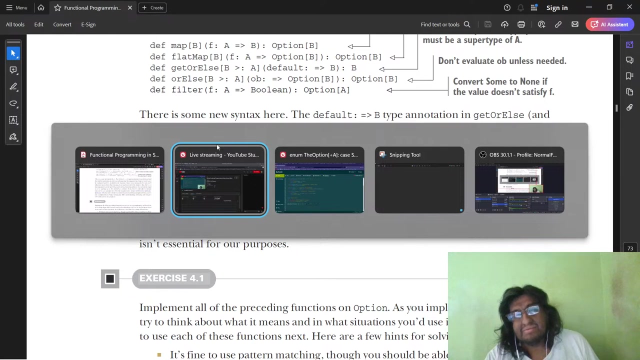 the last little one in- i don't want to say little one- the last exercise- i don't want to classify this- the last function in this exercise. okay, see you tomorrow with, or else okay and bye. thank you very much, or i can. okay, bye you.